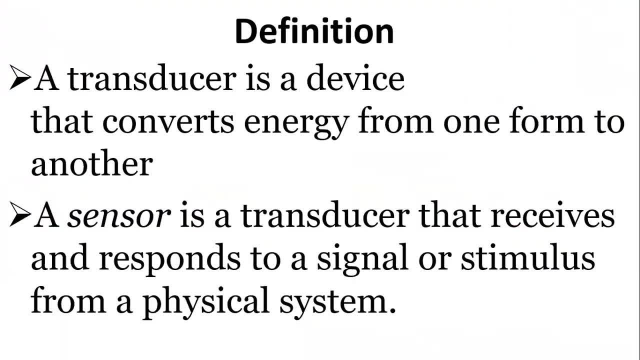 So let's understand the definition per se. To see the definition, a transducer is a device that converts energy from one form to another, One physical form to another form. So pressure to electricity, electricity to pressure, mechanical to chemical, chemical to mechanical. 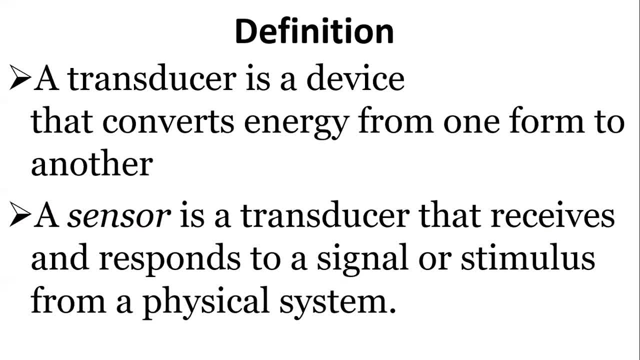 So one form of energy into another form of energy, Whereas a sensor is a transducer in itself that receives and responds to a signal or stimulus from a physical system. It just receives some response from the physical system. That's why we normally call it as a sensor. 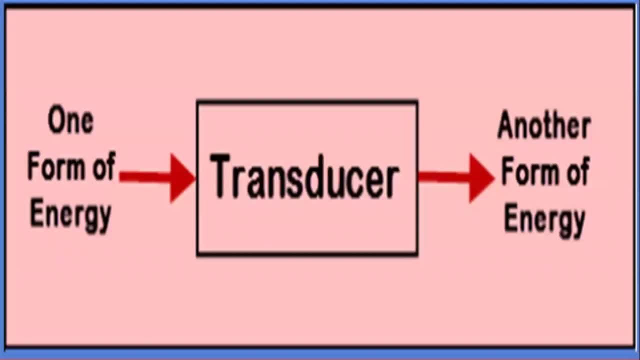 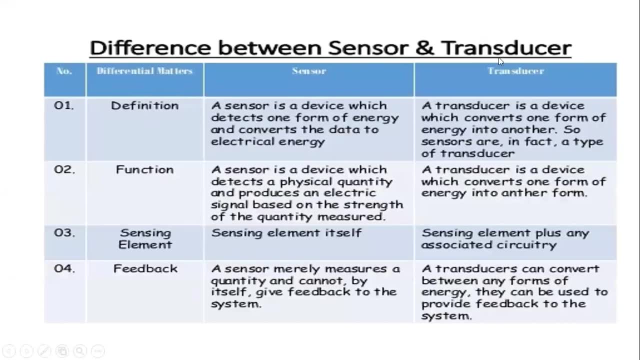 Let's get into it, Let's go slightly deeper into this. So, basically, a transducer converts one form of energy into another form of energy. If you see the slight difference between sensor and transducer. if you see the definition itself, a sensor is a device which detects one form of energy and converts the data to electrical energy. 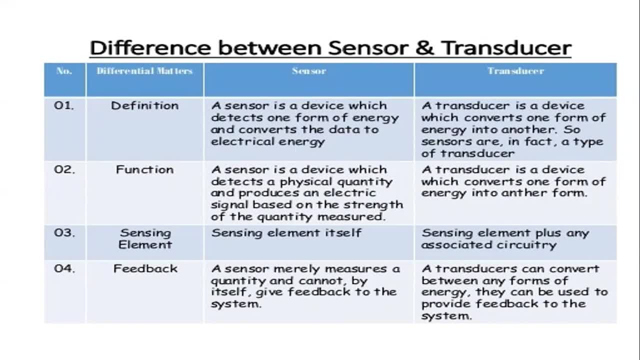 So lower values, lower magnitudes, lower amplitudes of electrical signals, electrical output. if you are getting from a device, And that we know, We normally call it as a. to be specific, we call it as a sensor, whereas a transducer is a device which converts one form of energy into another, as we have seen earlier. 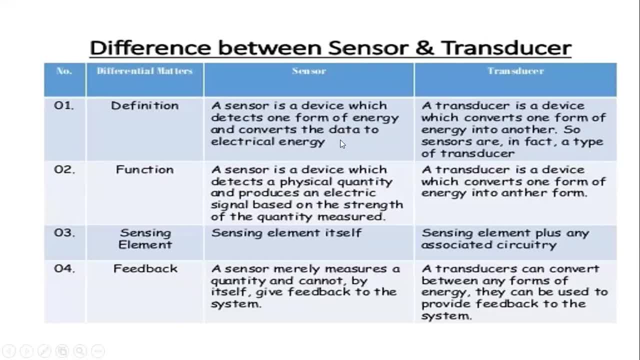 So sensors are in fact a type of transducer. So if the signals available are of very low electrical energy, we normally call them as sensor. That's as good as that. And if you see the function wise, the sensor is a device which detects a physical quantity and produces an electrical signal. 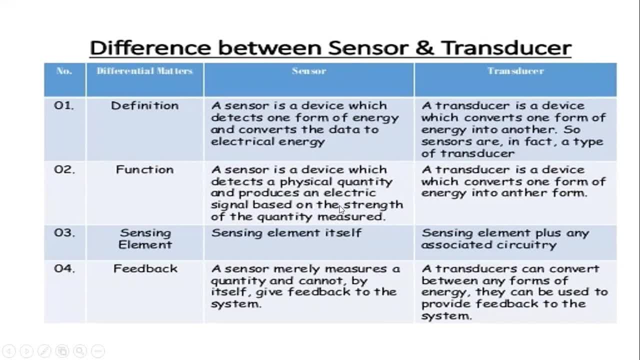 Based on the strength of the measured quantity. we normally call it as a measure, and quantity that's being measured is called, termed as measure, and so that is exactly what is the function of a sensor, Whereas a transducer is a device which converts one form of energy into another form. 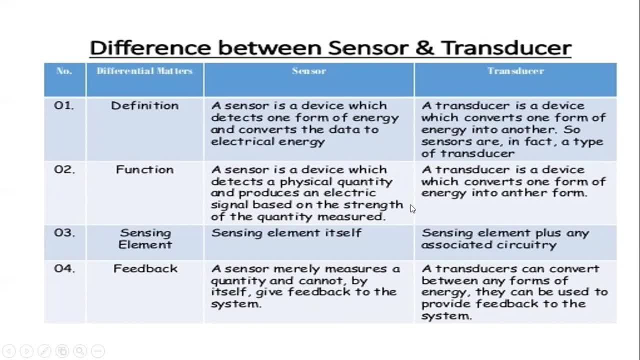 Basically, the definition and function are more correlated. in that way, Then the sensing element is the sensing element itself, Whereas a transducer is sensing element plus some associated circuitry. there could be some other transducing part of it after sensing the thing, because the the output of the sensor is always a very, very low. input. electrical output, electrical signal. 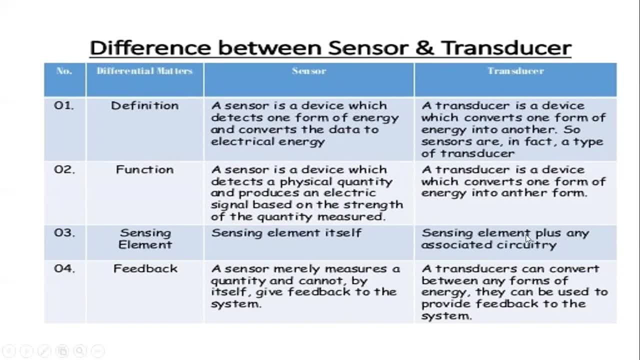 And that has to be suitably converted to a stage where it can be detected by the signal conditioning system. This we will understand when we come to the role of the transducer. then, when it comes to the feedback, both can be used and cannot by itself. 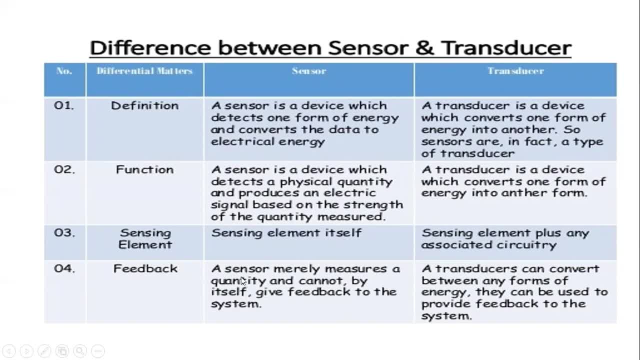 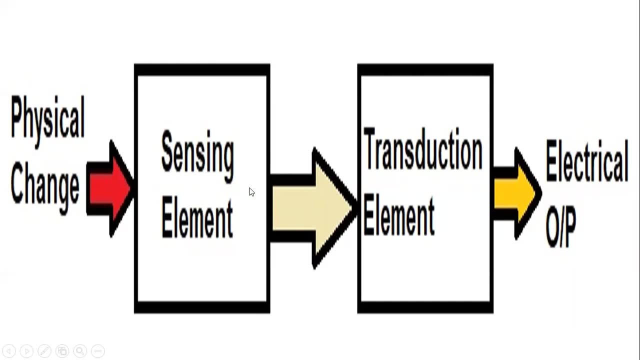 You feedback to the system as a sensor, but whereas a transducer can be more conveniently used as a feedback element in any control system. So a physical change is normally sensing, the physical change is giving a very light signal and where you have another transaction element to convert it into electrical output, 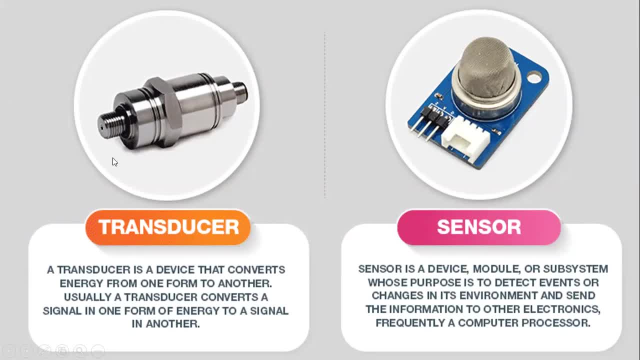 So these are the typical examples. we have a typical transducer measurement. They look like this. a typical sensor may look like this. So again, a transducer. usually it converts the signal from one form of into another form that we have seen, whereas here is it can be a module, or it can be a device, or it can be a subsystem. 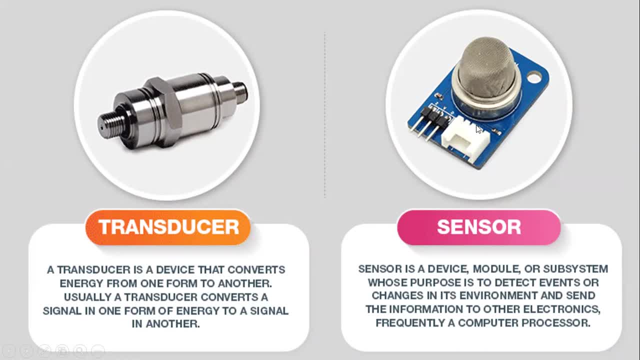 For the purpose of which is basically to detect the events or changes in its environment and send the information to other electronics, frequently a computer processor. It can be a little, because the output of the sensor is always a low electrical signal. That's exactly. is the definition by difference of transducer and sensor. 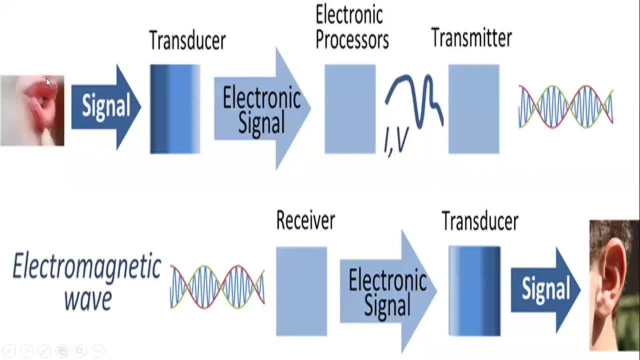 If you take a typical example to understand the signal, we have a, an audio signal which is coming, a transducer which is converting into a electronic signal, and then you have electronic processors- signal conditioning, we normally call it- and then it is transmitter transmitting to a longer distance. 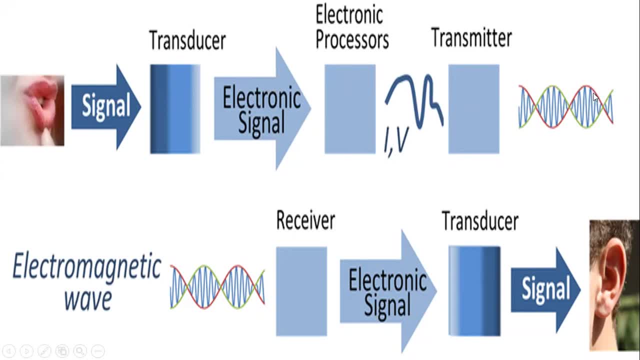 Normally call it as a telemetry- in the form of electromagnetic waves. right now, these electromagnetic waves are received by a receiver which is nothing but an electronic circuitry, The capacitor Gantt. then this cell converts into electrical electronic signal. this electronic signal is converted back by a given transducer from electronic to audio signal and that signal we normally listen. 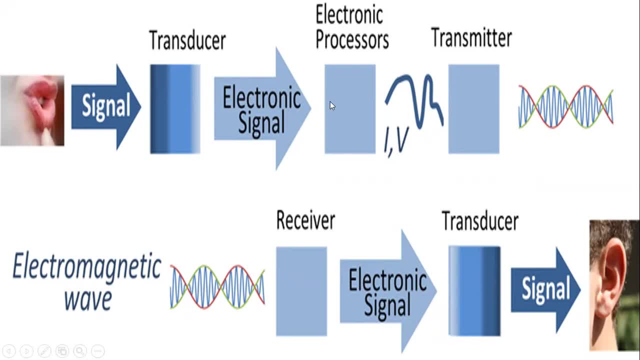 So, if you see, the audio signal is getting converted into an electrical signal. It's being transmitted to far of distances, again received by another receiver, and then electronic signal is get again- the transducer. here. this transducer is converting audio signal into electronic signal, Whereas this transducer is converting electronic signal into audio signal. So that's the exact role of the sensors and transducers in a typical application. 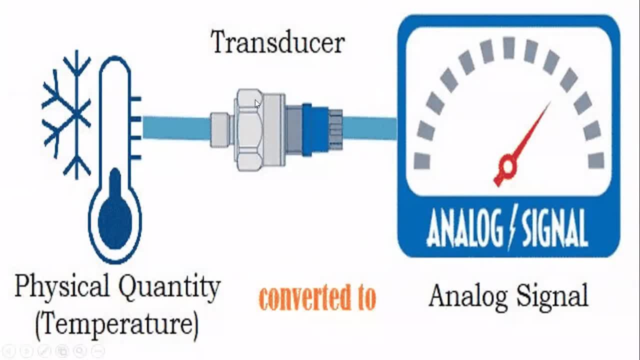 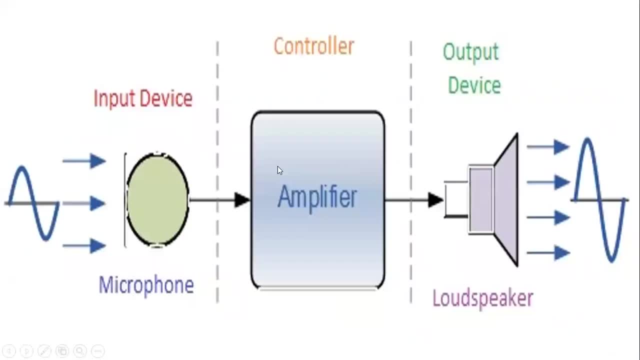 Then again you have a physical quantity which is being converted, Converted by a transducer into an analog signal which is being read here. This can be another example. Right, This is another example which we have seen: a microphone- typical microphone- is an input device, whatever thing. then it is given to an amplifier and it's then loudspeaker is an output device because this amplifies the signal- little low magnitude signal that is getting. then it is given to the loudspeaker and here it is basically the amplified signal, the same. 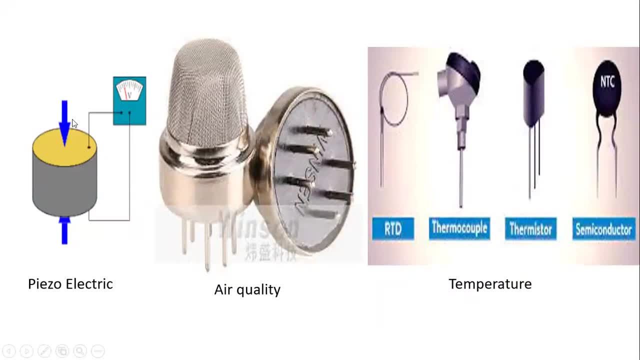 These are the typical examples. we have a piece of electric sensors. you know, pressure to electrical signal. when we apply a compressive force here, Now we get the Electric charge that we can easily read it here. So this air quality measurement sensor. Then we have temperature sensors, RTD resistance, temperature detector. Then we have a thermocouple and we have a thermistor and semiconductor. All these are the. 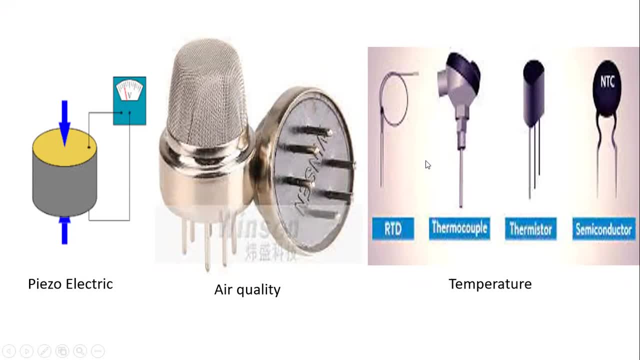 What you are, которое we call them three ideas. These are the transducers which give the electrical output, So for all practical purposes we can call them a sensors, also Freeze, Let's say. that is basically the ridiculously quiet reference we have. 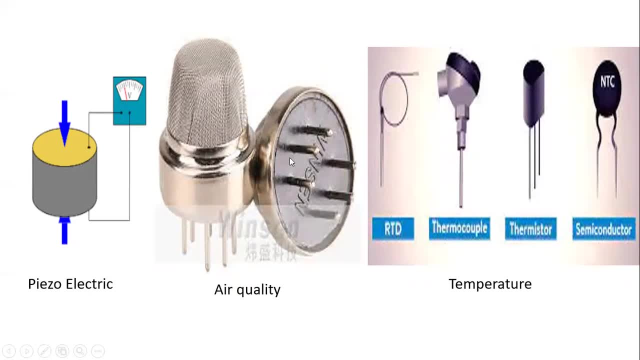 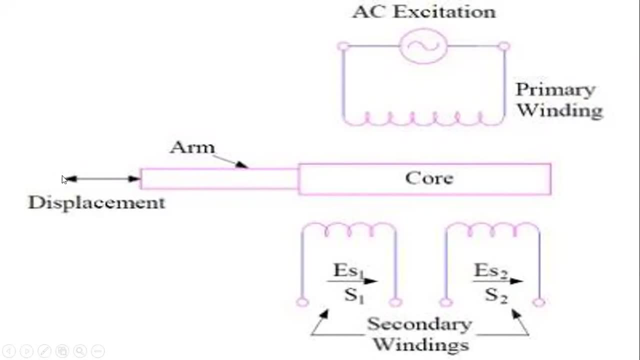 Right. So that is the basic DIffrenc AC4 of these. so this is a typical linear variable differential transformer LVDTV, normally co- The Difference: when we display the Electric signal格ague čgtakãr, we excite the primary winding, the output that we are getting at the secondary winding is 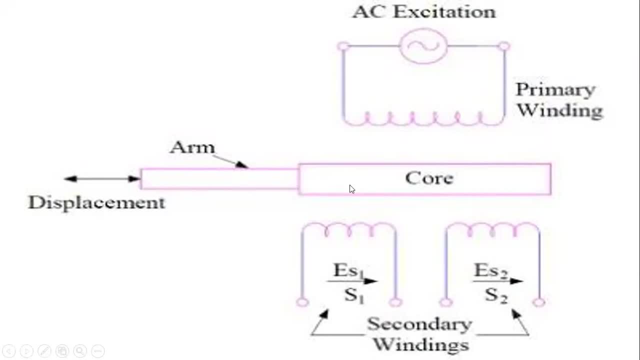 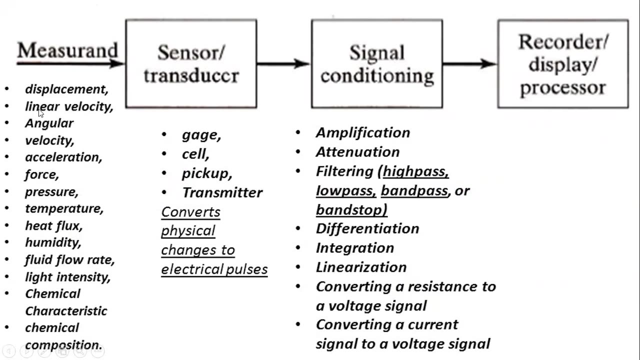 proportional to the displacement of the core. Okay, this is a typical principle of a transducer, where we are getting. And then, if you see the typical measurements, all these parameters: displacement, linear velocity, angular velocity, acceleration force, pressure, temperature.